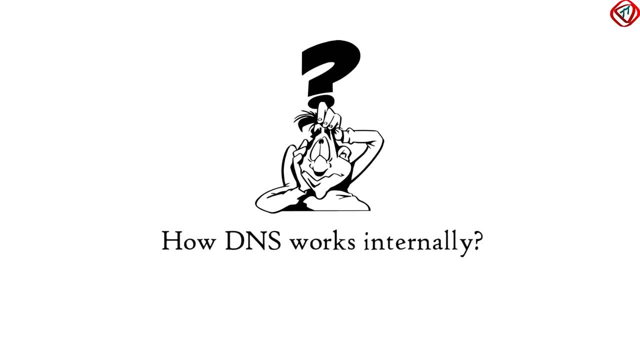 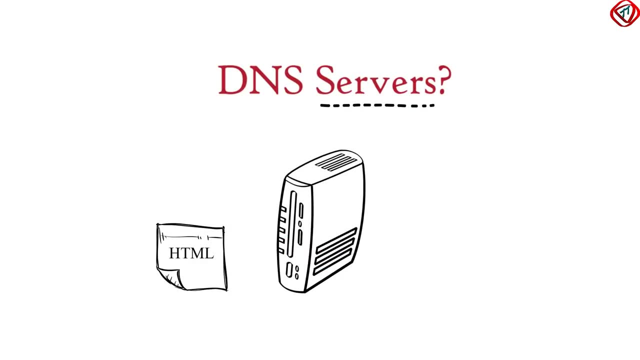 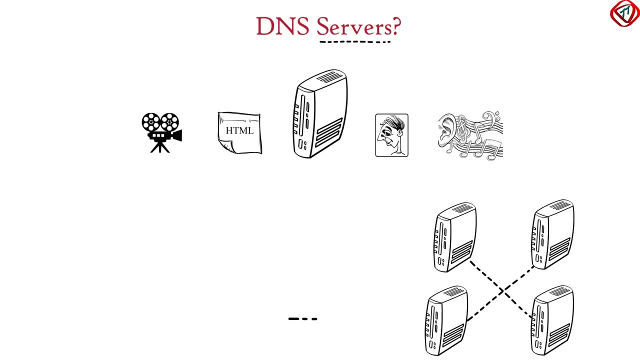 So how DNS works internally. To understand this, we should know what are DNS servers. Servers are computers storing HTML files, images, sounds, videos or any other file types. Servers that work together to provide IP address of the requested website to the web browser. 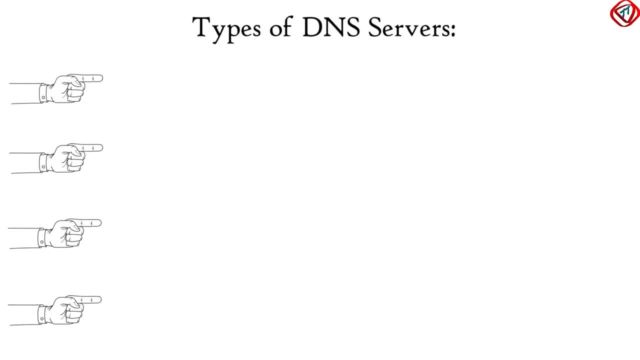 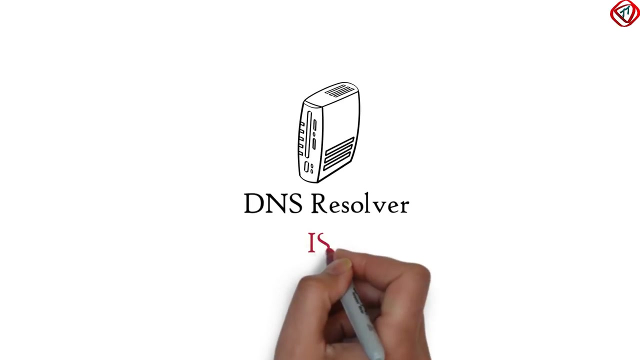 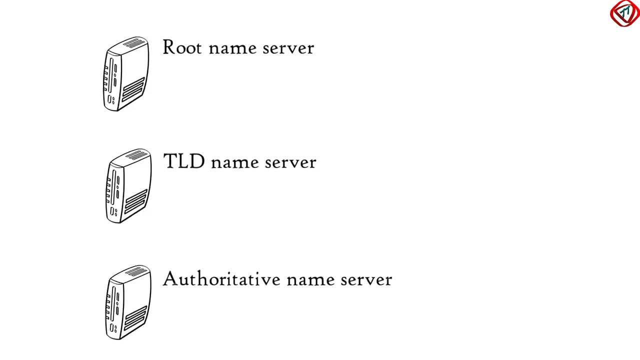 are called DNS servers. There are four types of DNS servers: DNS recursive resolver or DNS resolver, root name server, top-level domain or TLD name server and authoritative name server. DNS resolver is provided by the internet service provider. It connects the web browser of our computer to the DNS name servers. There are 13 sets of root name servers. 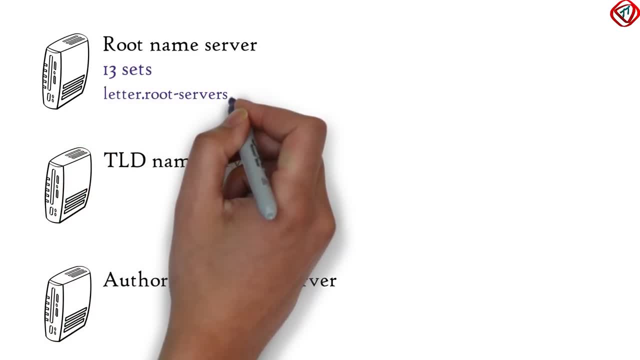 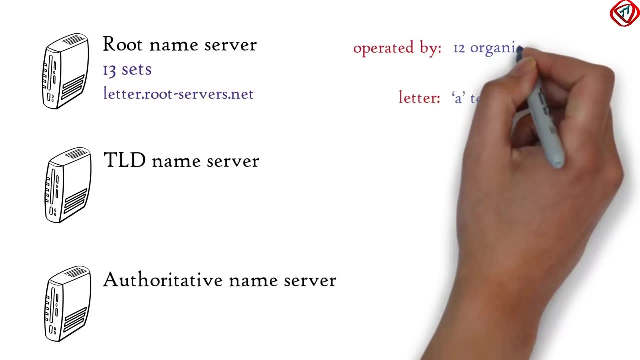 logically named as letter dot file, Letter dot root dash servers dot net, where letter ranges from A to M and are operated by 12 different organizations. Each set has a number of servers placed around the world. 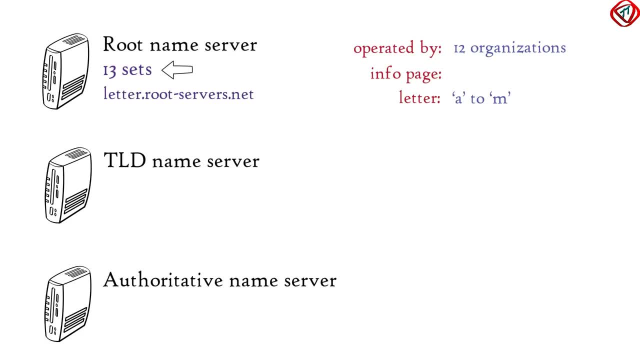 An informational page exists for all root name servers at address letter dot root dash servers dot org. where letter ranges from A to M except G For G. this is the home page at which this serves. Details of all root name servers can be found in the. 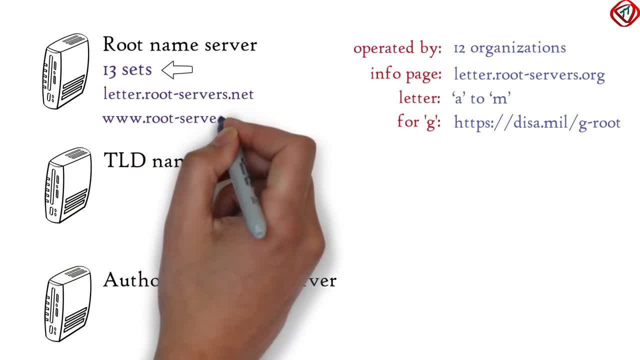 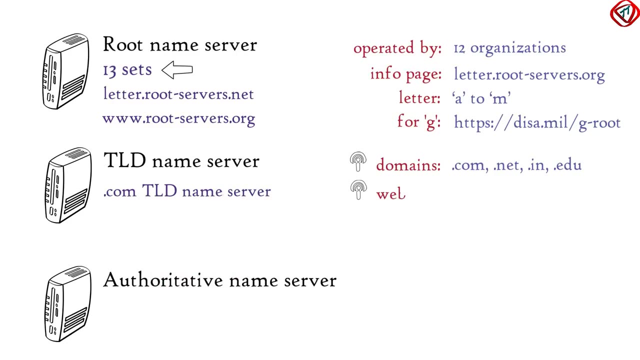 website: wwwroot dash servers dot org. TLD name server stores the information of all domains sharing a common domain extension, For example, com stores the information of all websites ending with com. net name server stores the information of all Web sites ending with: 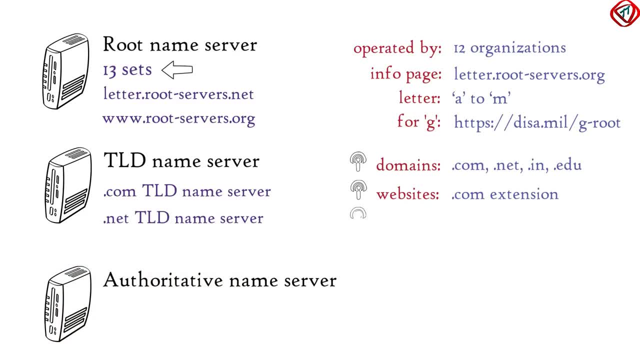 ether and runners we have use the open source. com is a means ofei utility machines etc. Also, the one tool use by which we find com isas pane independent to Internet user net iso ableų channel, that is, Internet Cooler. 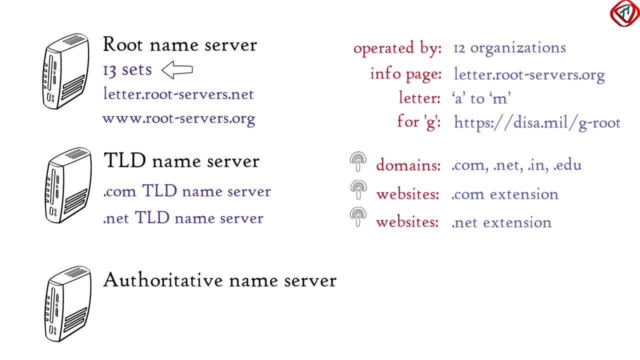 ReadAlum and others where assassination is accepted. TLD name server, The working Names server, is a master purported of all NET websites, and so on. Authoritative name server is the last server in the domain name system. It stores the IP address of the requested website. 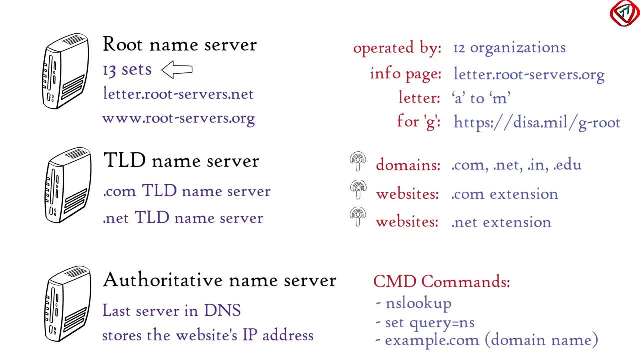 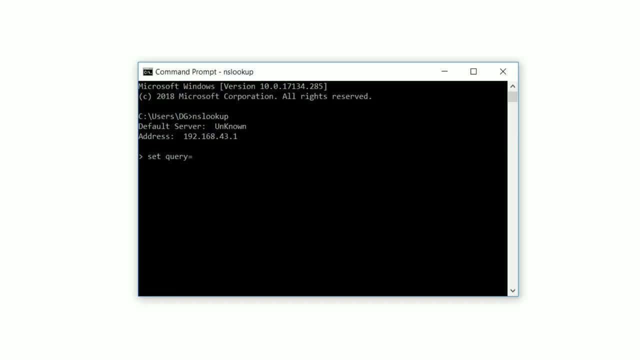 Authoritative name server for a website can be found with these cmd commands: Open cmd and type nslookup. hit enter. Set query equals ns and hit enter. Then type the domain name. hit enter. You will be able to see the authoritative name servers. 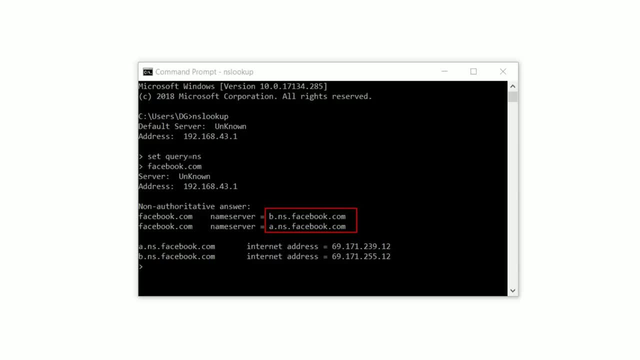 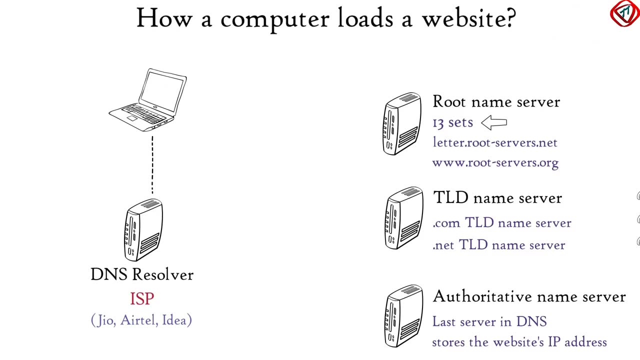 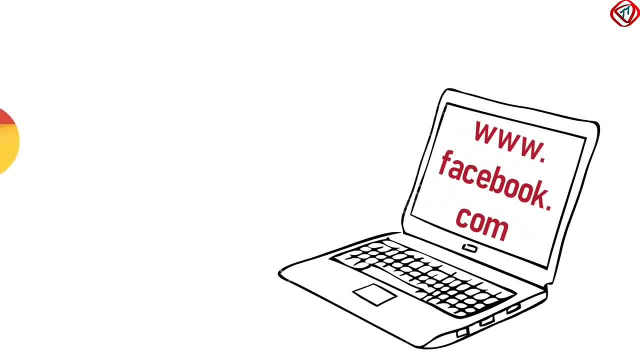 One is master and the other is slave. Slave is the exact replica of master and is used to share the DNS server. load Now how a computer loads a website. Suppose we type facebookcom in the web browser. Since web browser needs IP address, so it forwards the query to the computer's operating. 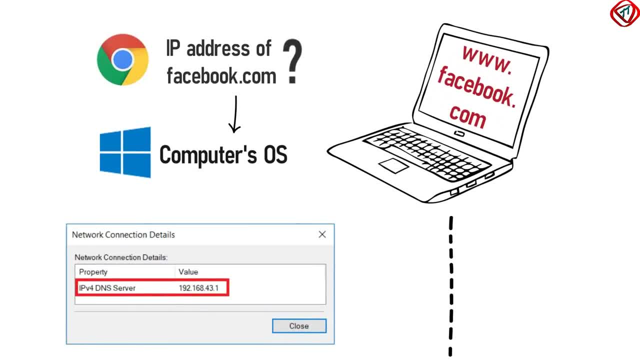 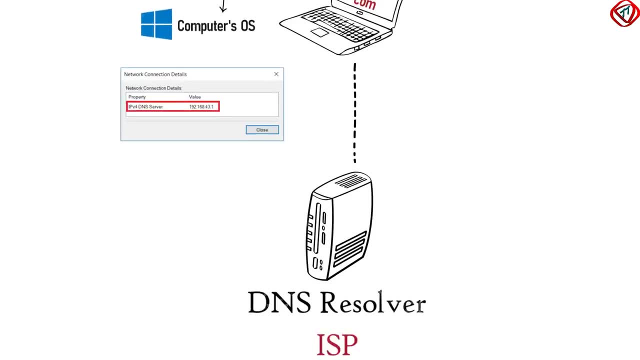 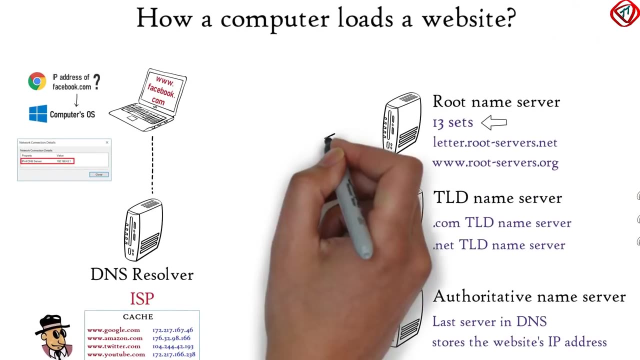 system Operating systems are configured to forward the query to the DNS resolver Operating system then contacts the DNS resolver. DNS resolver checks its cache whether it has the IP address of the requested website. If not, DNS query is forwarded to the root name servers. 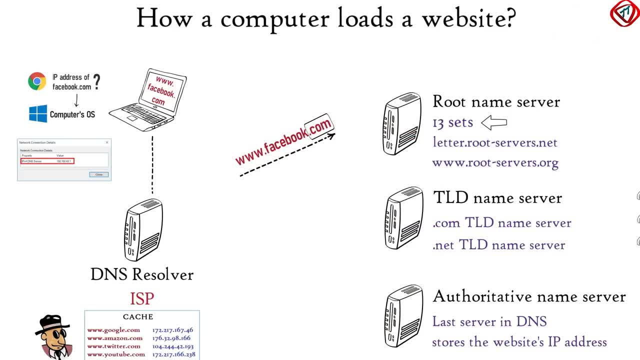 Root name server checks the extension of the website, whether it is com, org, net, in, etc. Based on the extension, the root name server provides the IP address to the DNS server. The root name server then checks the extension of the website, whether it is com, org, net. 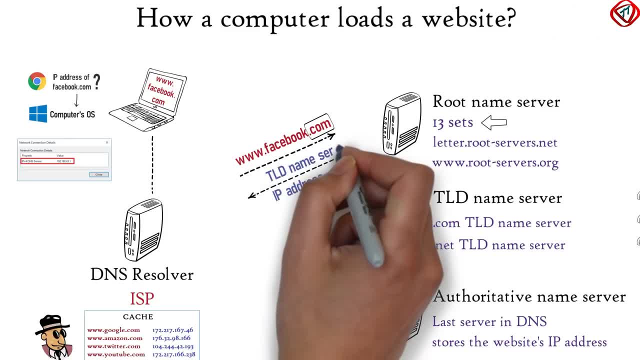 in, etc. stattThe IP address of TLD name server to the DNS resolver. DnsResolver converses with DNS server. IP address of the TLD name server is provided to the DNS resolver. DefenseTele terapist then checks it if one of the IPs is not current. 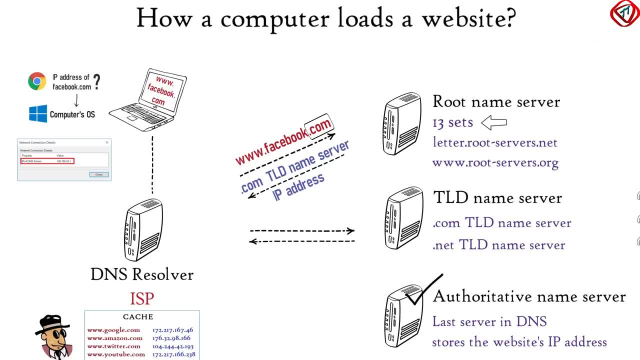 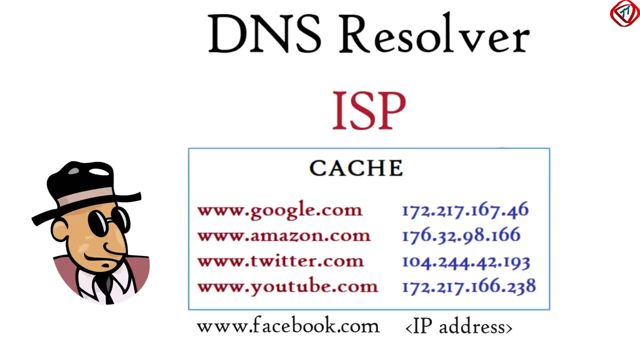 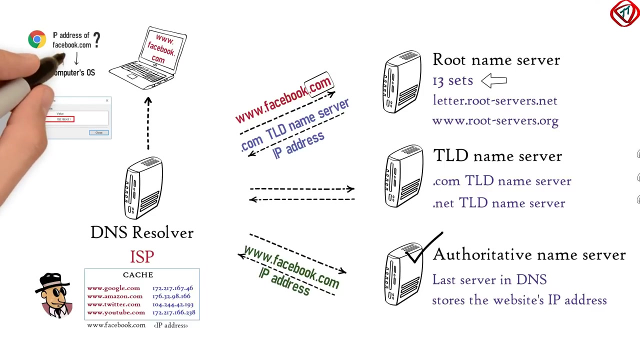 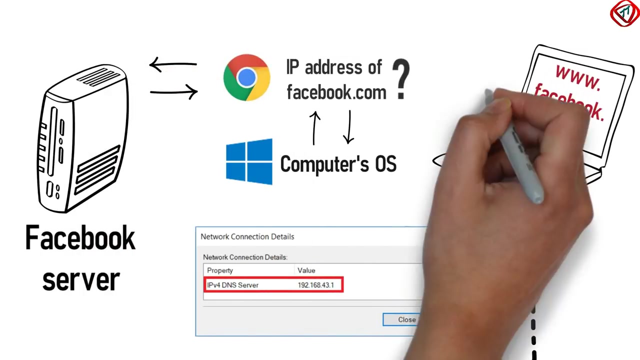 ayo, Which should necessarily store the IP address of the requested website. Finally, the ingen DNS resolver stores this information in its cache for future use and provides the IP address to the computer's operating system Operating system then forwards it to the web browser. The web browser then contacts the Facebook server and loads the requested website, ie. 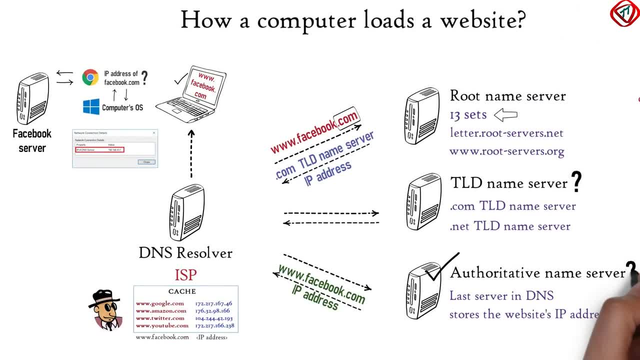 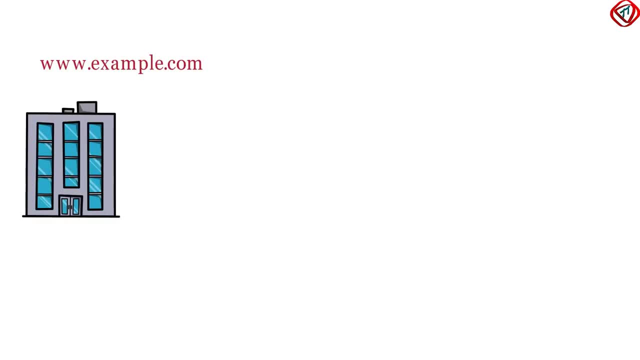 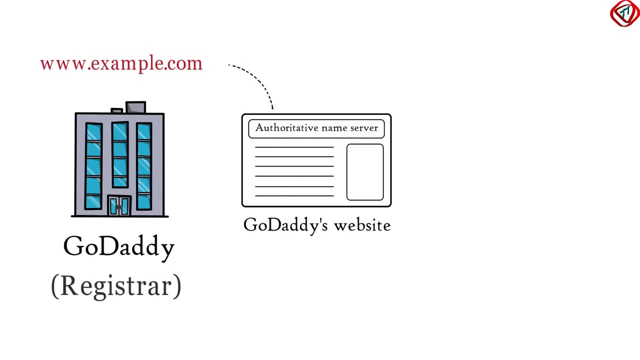 facebookcom, But how tld nameserver knows which authoritative nameserver stores the IP address of the requested website. It all begins when we purchase a domain name from a registrar, ie GoDaddy. In registrar's website we can set the authoritative nameserver that domain should use. 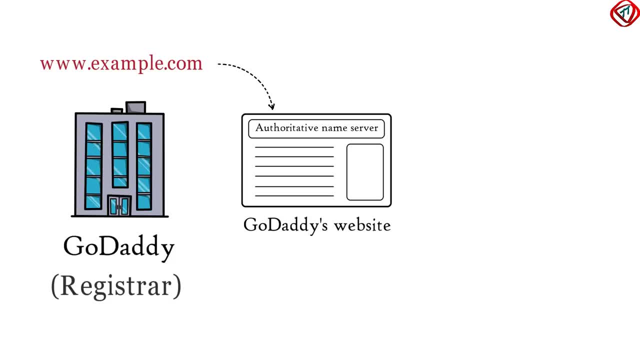 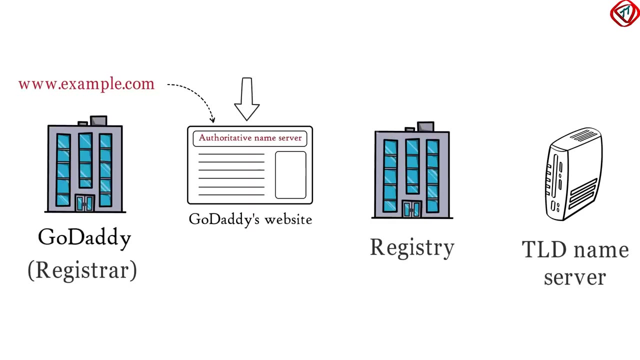 We get the details of authoritative nameserver when we buy a web hosting plan from companies like Hostgator. Once authoritative nameserver details are entered in the registrar's website, registrar tells the tld nameserver managing authority registry to update the tld nameserver and